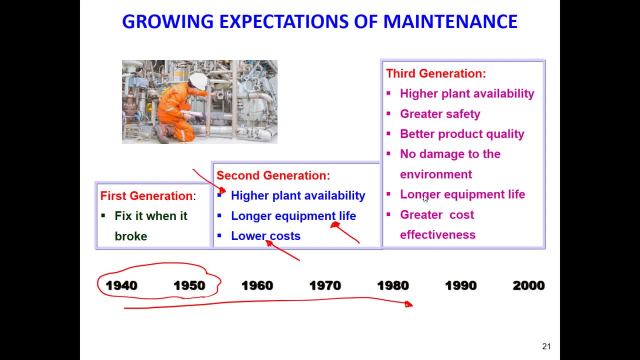 So they prepare the maintenance activities based on these objectives, And after that I mean the recent years, in the last 20, 30 years. so the maintenance has been much more accurate and it's been like a bigger activity that is aimed to reach to a higher planned availability. 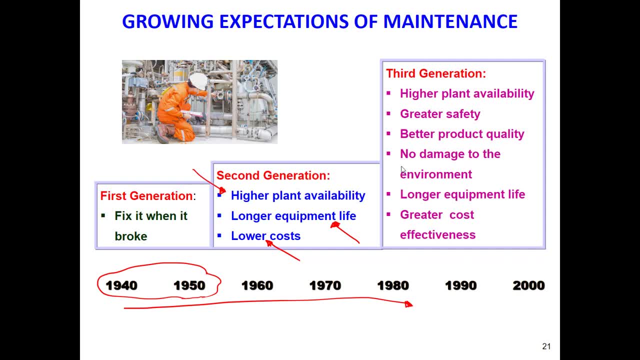 Better Safety, better product quality, no damage to environment, longer equipment life and also the less cost or more profit. Okay, so those are the things that is being considered. that is being considered when I mean for the maintenance activity in the recent year. 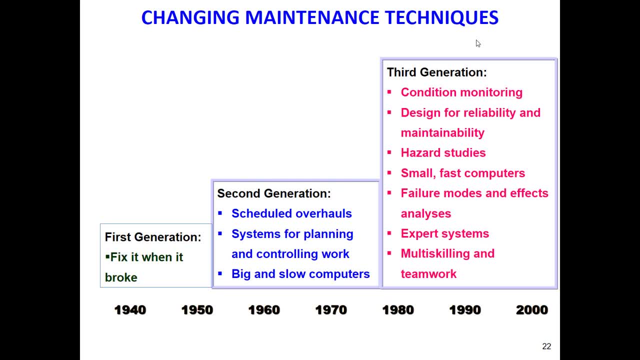 And okay. So The techniques, the technology that was used, okay, that has been used for this job has also changed. We had Okay, so before it was just fix it, Then in the first generation, fix it when it's broken in the second generation. you know they were some systematical and a schedule overall. 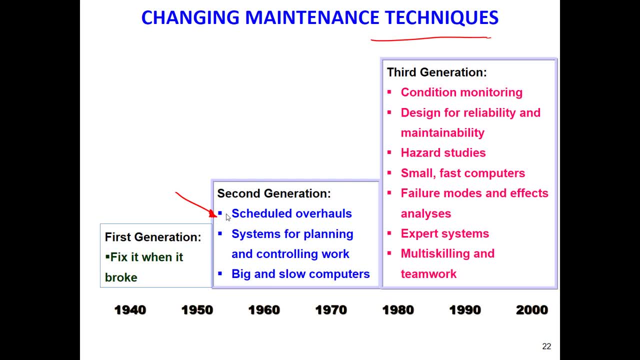 Overall means, you know, like, let's say, they were stopping this Changer after each few months and they were cleaning, fixing it and then putting it back in the operation. So that was the schedule overhaul system for planning and controlling work. 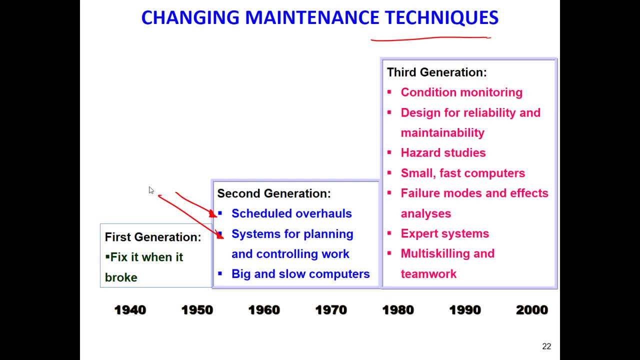 So like they had a work, you know like a systematic workflow, planning work and you know like for maintenance and also like computers. That was those times that they were big and slow. They also help for this maintenance thing. You know the schedule in the maintenance. but third generation, 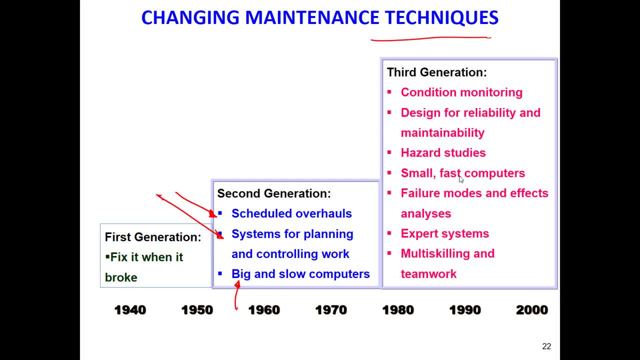 Okay, so in the third generation we had more and more technology, more instrument that we could monitor the condition of the equipment. Really, there were many technologies, software that you could design, you know, and they maintain the maintenance walls And there have been many hazard studies. 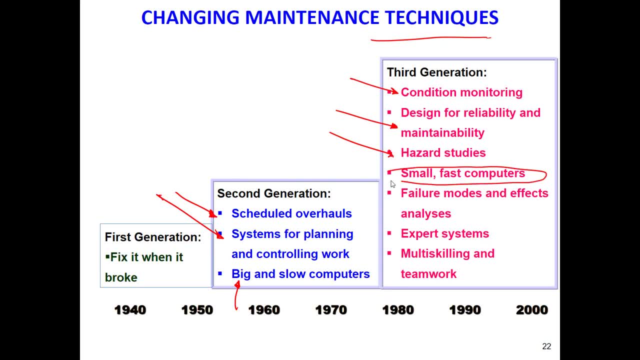 And they say we have very fast and small computers that can be used And there are many, you know. analysis like for for failure mode and face, you know, like a lot of simulation about that, A lot of expert systems. You know there are a lot of people that are expert in this job at this day. 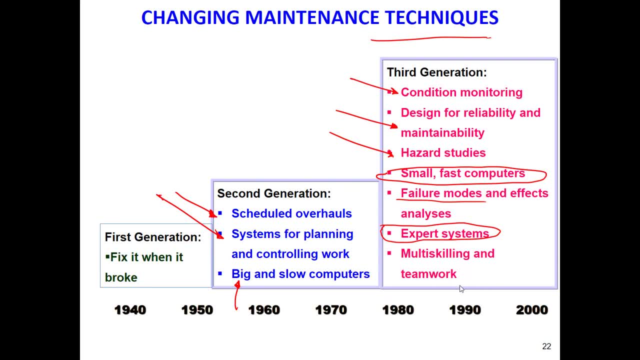 They have been educated in different you know and institutes, And also So what is killing? and teamwork, You know, like teamwork is also encouraged because maintenance is something that most of the workers. they have to be involved and collaborative to do it carefully. 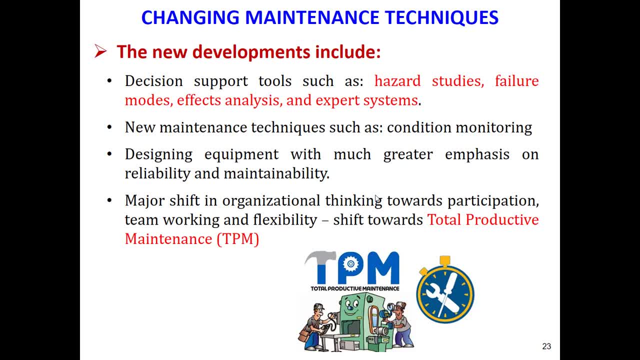 Okay, so the new development or the new new development or a new methods or technologies for for maintenance is aimed for For total productive maintenance, T, P, M or total productive maintenance. So that is considered To use tools for hazardous studies For the failure and effect mood and the failure mood analysis. 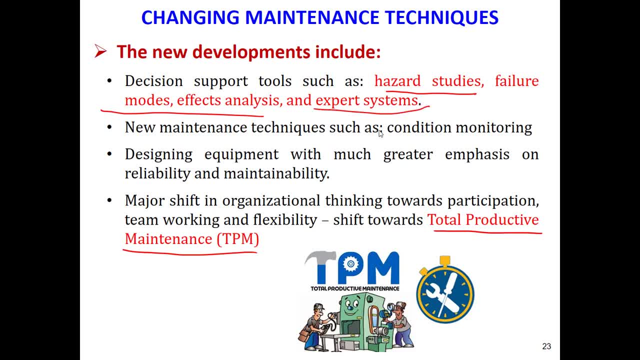 We are applying the expert systems. Condition monitoring is also new technology or new methods That you can monitor the condition of your equipment. It is in the good condition but condition It is working, is its maximum capacity or there is some issues? So you can really monitor. 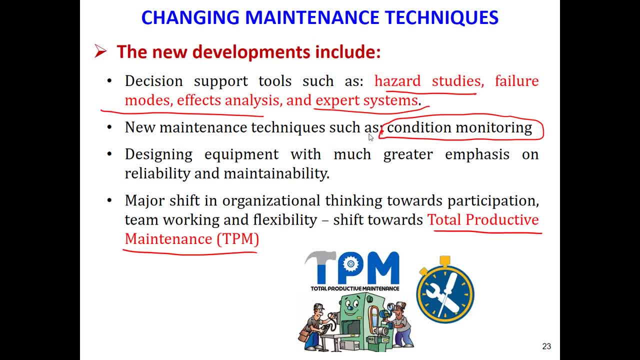 You don't have to wait until the equipment fail and then take some action. You can really monitor the condition of that equipment. Nowadays we have more technologies for fabrication, for construction, So we can design and build equipment With the best, With the better accuracy. 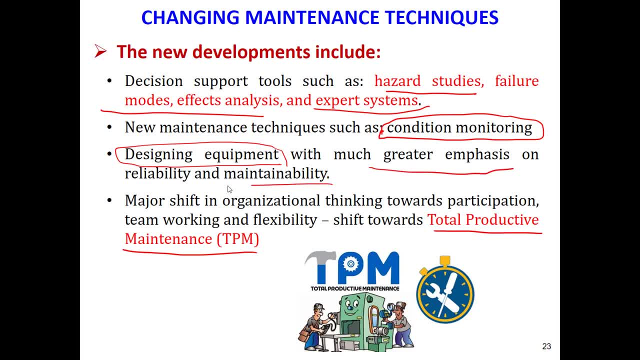 With the more emphasize on reliability and maintainability. Okay, so that's another thing, that for the design equipment And also, there has been a major shift from individual working or thinking to organizational thinking. Okay, organizational thinking by, by, by, you know, like encouraging the participation. 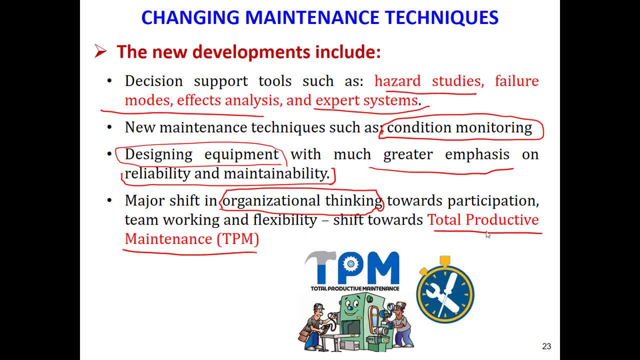 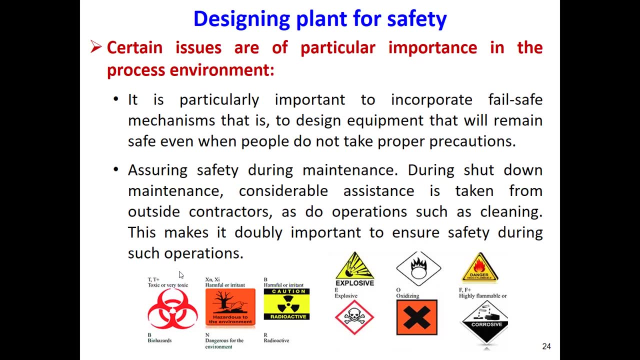 Team working and being flexible, That is, all of these activities is aimed to lead to a total productive maintenance, or TPN. Okay, so about also designing. So designing the plant is also- you know, when we are designing the plant- The design equipment. 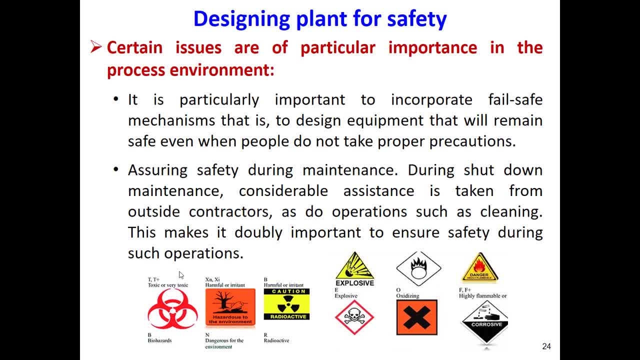 There is one, one phrase that is saying that designing plan for safety. You know it's very important that even if the in the plant there are some equipment that they fail, Or if there is a maintenance work is going on, So the plant is still safe. 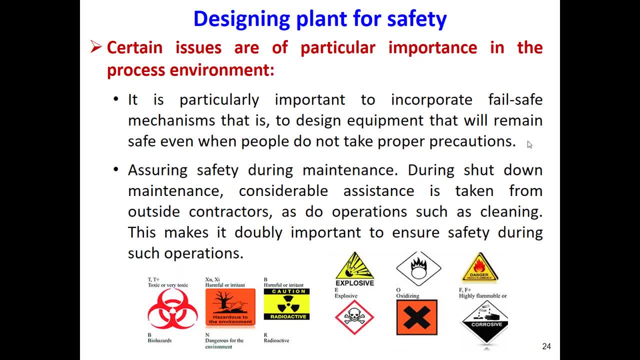 Okay, So there are. You might hear this term fail safe. Okay, fail safe mechanism is that the equipment, It has been designed in the way that, even if it's failed, the process will be safe, The equipment will be safe. That, as I said, one of the example how we can make sure the felt safe mechanism. 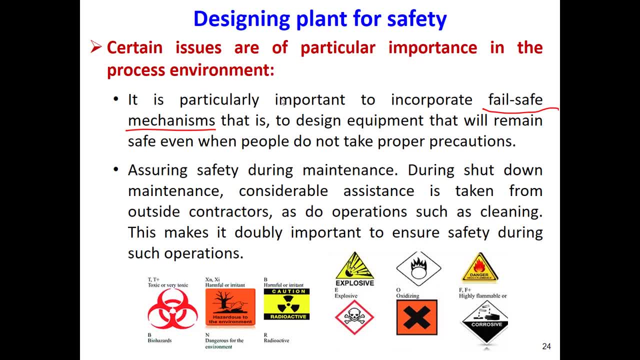 Let's say designing some switch, emergency valve, Some pressure pressure with the relief system, This kind of system They are help us to, to, to reach to such a, Such a mechanism. Then, during the maintenance- Okay, When there is a shutdown for maintenance- we have to also make sure that the process is safe to do the maintenance. 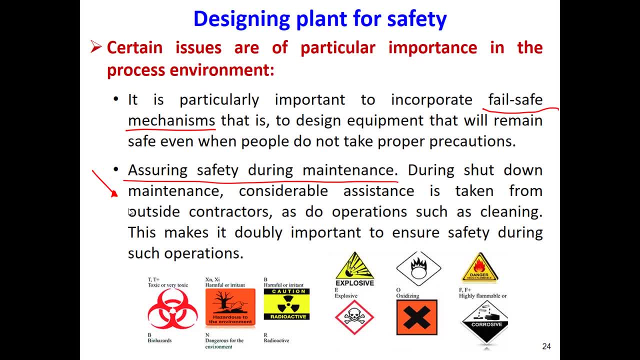 Let's say, sometimes you have, you have the equipment that you need to clean it, So you will commission that to outside. You will, you will bring a contractor from outside, like a company That is expert in cleaning, to clean that equipment. So you have to make sure that the process is safe for them to come and do the cleaning. 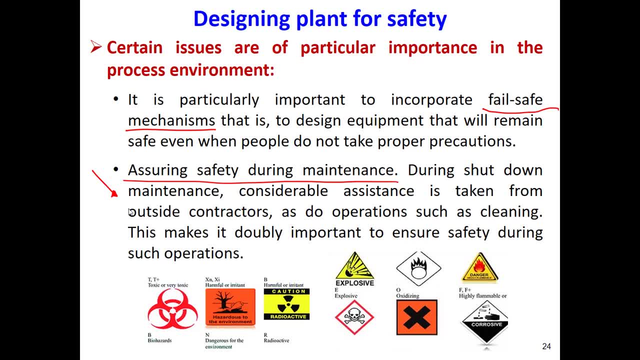 The maintenance work is also being done safely. Okay. So like there are many cases of you know like really catastrophic, catastrophic accidents that let's say, they stop one equipment and they start doing the maintenance. They didn't think Really Maybe the effect of that stopping that equipment or that maintenance to the other part of the plant that that led to really, you know, like explosion or, you know, to a very bad accident. 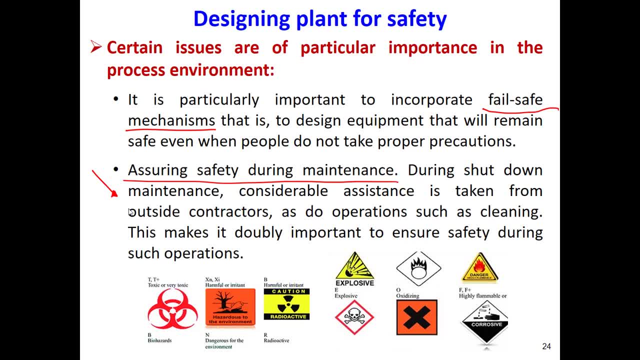 There are many cases, you know, if you just search in Internet, YouTube, you might, you might find, you know those cases. Not like in aviation industry, you know, for the maintenance is a very important part. So the maintenance is done on the aircraft. 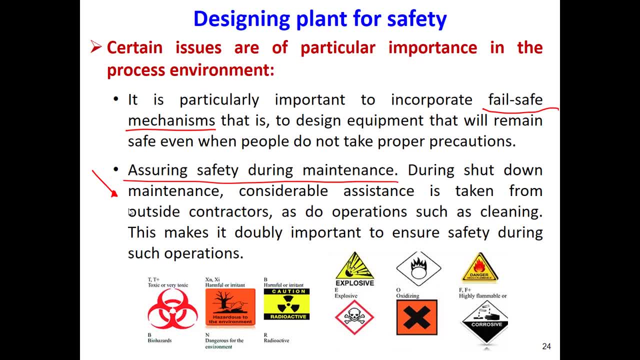 Usually when they land, there is a protocol to maintain the, to check many things in the aircraft. So, like, once they they do the maintenance, the overhaul, they have to submit a very accurate, precise report to their managers or the pilots. So to make sure that the aircraft is safe to to, to, to take off or, you know, to work again. 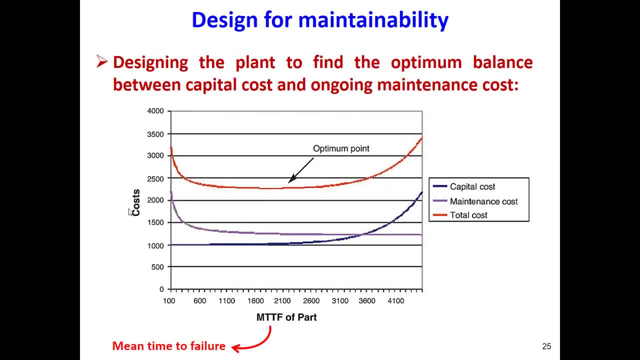 So those are some points We need to consider. Okay, So then, when it comes to the maintenance, maintainability, I mean, like one question is always: what's the optimum age of of equipment or a part to be used in the process? 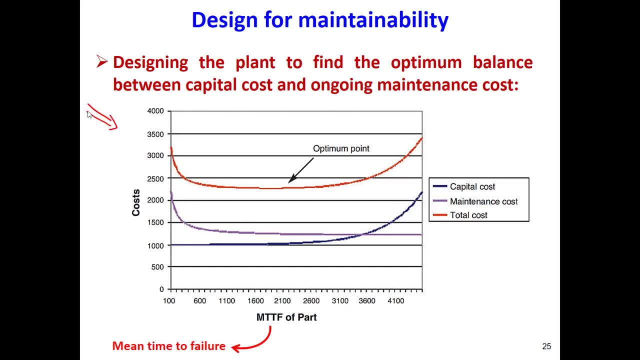 Okay, There are to do that, to find the optimum age of a part of equipment. in the process, There is always such a curve Like that that can be used by the designer, by the managers, to to make some decisions. What is this curve? 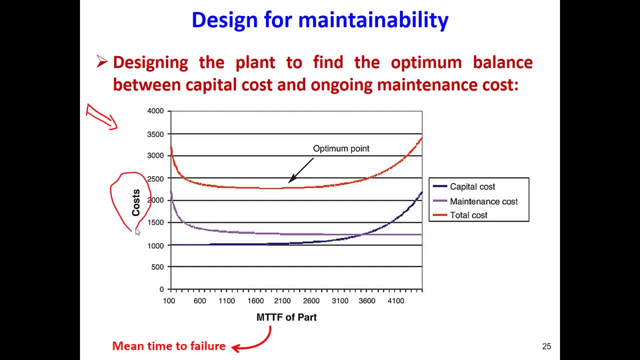 So you have in the Y axis you have costs. in the X axis You have MTF of the part of equipment. What is MTF is mean time to fail. So it can be, let's say, days, usually days. It can be days. 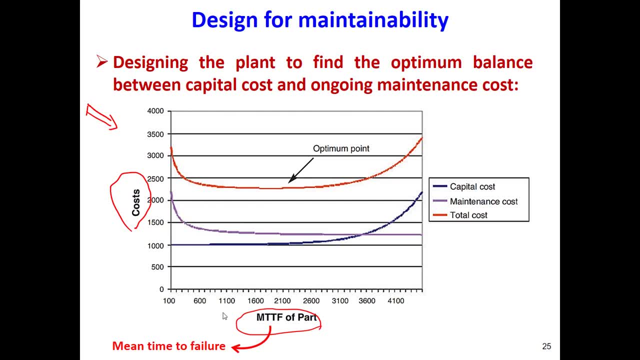 It can be weeks, It can be years. So you have, So you have mean time to fail. It's the time that that equipment, that part will fail. So for that part the capital cost, usually at early age, early days, early years is is, is not increasing because, let's say, inflation is constant. 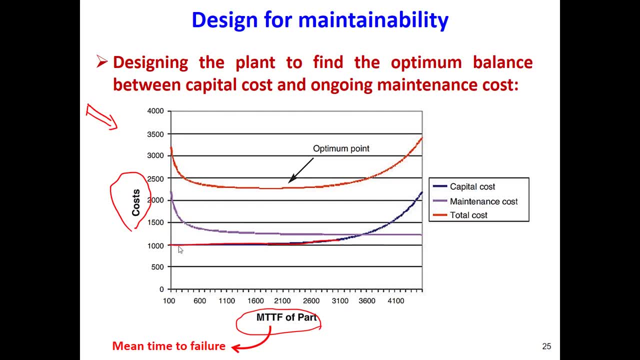 So you buy that part, that equipment, you will install it, So you don't pay really any money Until that part starts to you know. let's say, if it's a compressor, So you need to repair the compressor continuously, You need to change the parts. 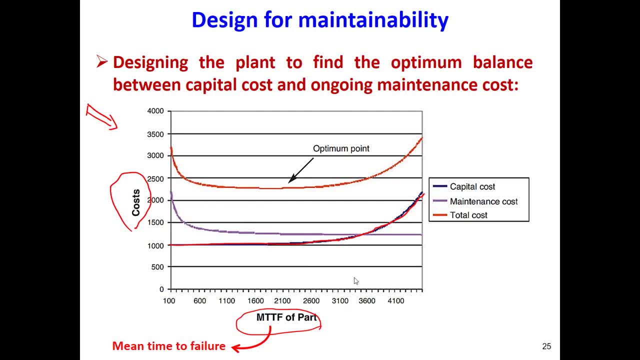 You need to do a lot of. you need to change the parts of that compressor or something. You need to change the motor, the driver, the shaft, So that increase your- I mean that increase your- your cost of that equipment Once it's you know, you start using it after a few months. 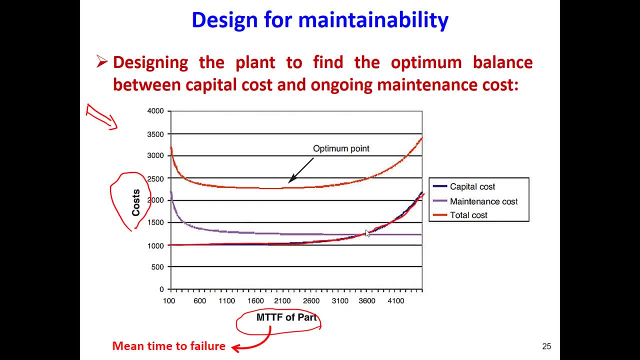 After a few years it starts to become costly for you. It's like a machine, like a car that gets old. It has more money to change. You know you have to change different parts. You have to change the. you have to change, you know- the tire. 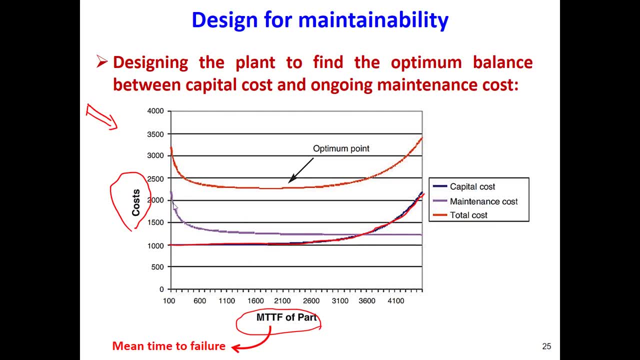 This kind of thing. that is usually capital maintenance. So the equipment you know once are in a solid at the beginning, they need a good maintenance. You know like, because you need to, You need to fix a lot of things. You need to, you know like, change the oil. 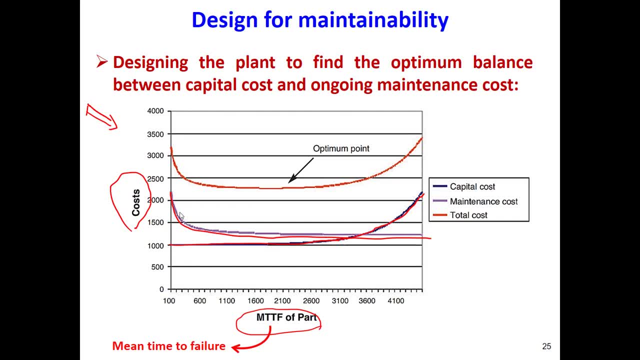 Let's say continuously: You need to make there is no leakage, continue. So at the beginning it has some kind of maintenance cost And but as long as it's- you know like it start working, the maintenance cost will be less. 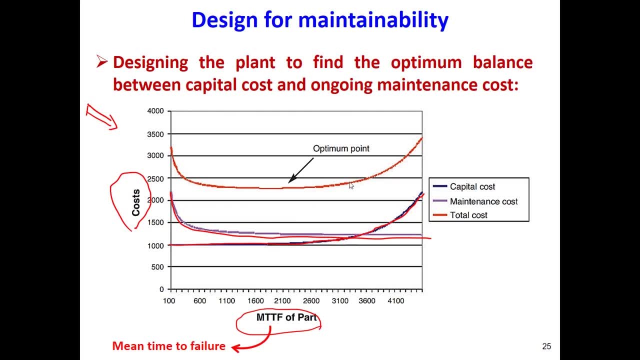 But capital cost might increase. There is a point, There is a age, There is a range that this total cost, Which is the of the maintenance and capital cost, will be minimized Like, let's say, this range: That is a minimum total cost. 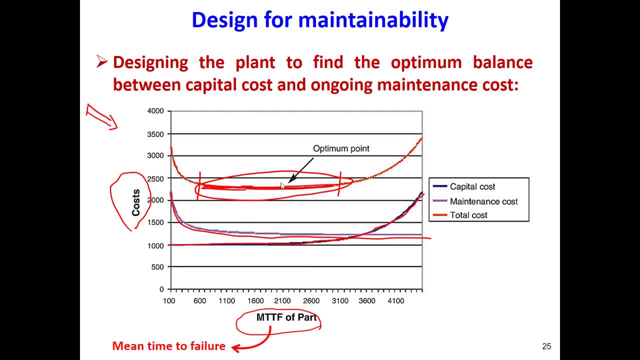 So is this, this range, Tell us the best is the range that we can use that equipment or that part in the best way. is the best time of range, Range of time that that equipment or that part can be used? out of this one, You can see that the total cost will be more. 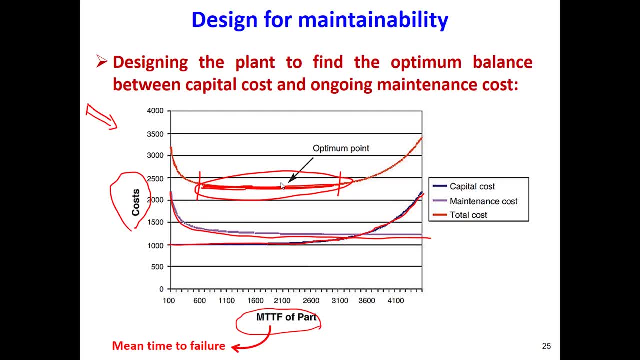 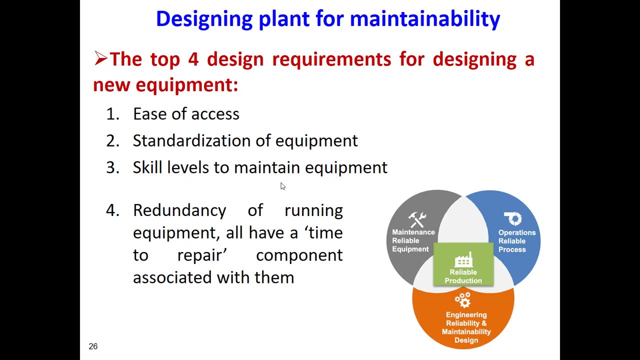 So we have usually such a such a curve, such a graph, such a tools to be used for for maintenance job, And I mean evaluating the maintenance and the cost of the equipment, Designing the plan for the maintainability. So when we are designing a plan there is kind of four design requirements. 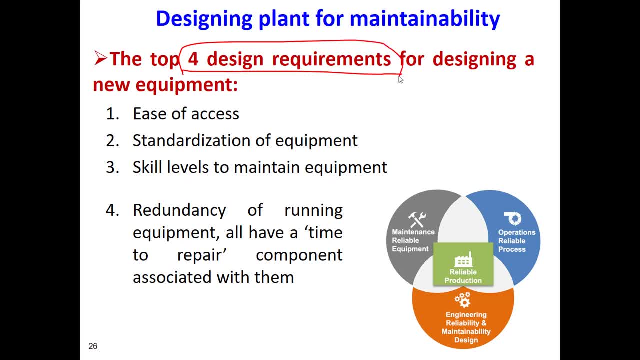 For the maintainability. For the maintainability, there is four requirements. First, easy to access. Each equipment should be easily accessible. We should be able to have to access to them easily to repair them, to change them, to replace them. 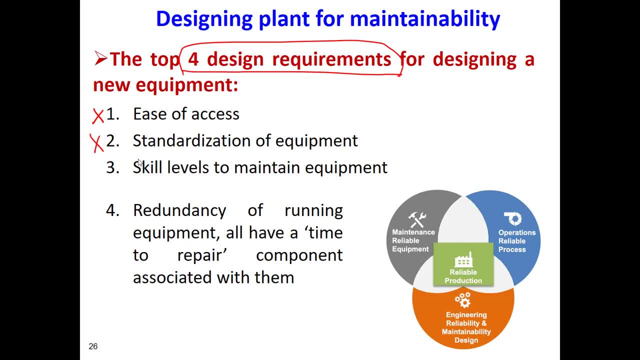 Standardization of equipment. So all the equipment they have to be work working in the standard condition, The standard design condition. We have to evaluate what is the skill level that is needed to maintain that equipment. Okay, this also we need to evaluate this. 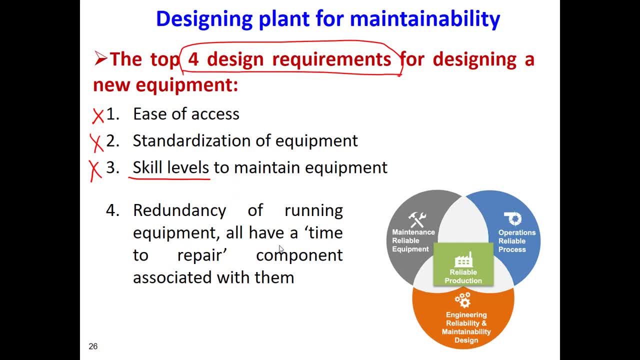 We need to report this- and also redundancy of running equipment. Okay, so we have to. we have to evaluate, like after how many months or after how many years we expect to repair or replace that equipment. Okay, Those are the four important things that we have to consider when we are designing the equipment. 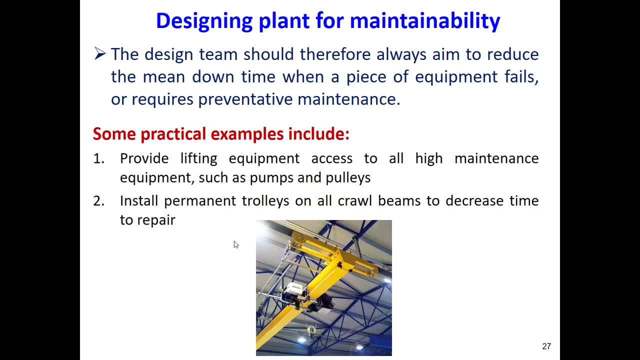 Okay, one example Like one example, for example. So, first of all, we have to always we have to minimize the time that the equipment will fail. We have to try to design or choose the equipment that will be failing. I mean the minimum way. 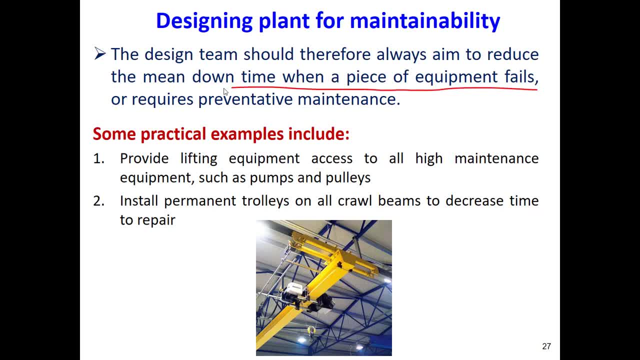 I mean like minimum time. I mean, let's say, minimum time per year or per month. Okay, so equipment has to be designed to work continuously and to be reliable. So we have, we need minimum maintenance, need minimum cost for maintenance, And okay, some example is, let's say, for example, for pump compressor. 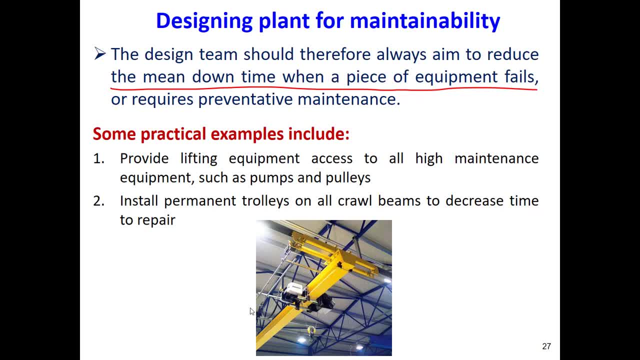 Those are the equipment that they need. They continuously need maintenance heat exchanger, So we need to, for example, for accessibility, we need to design such a lifting, you know, devices close to that equipment. You know we have to make sure that we have, kind of, you know, like we have already planned and installed some instruments, some devices that we can use to move that equipment. 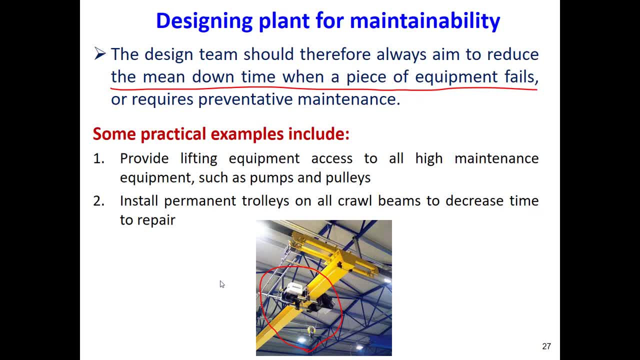 We can lift that equipment, put somewhere else, Bring another new equipment, replace it, do the repair. So those are the things that need to be considered when we are designing the plant. Those are the details that has to be really considered carefully. 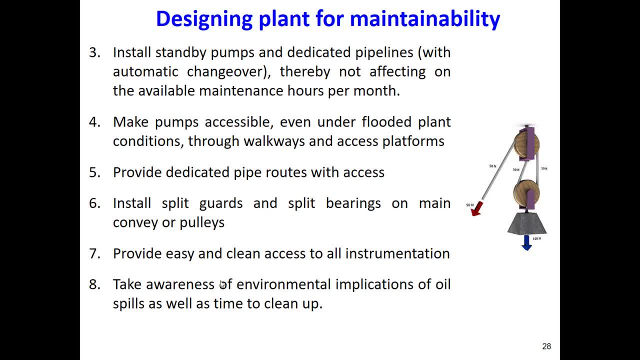 Then okay, those are also some additional points about designing a process For maintenance. So we have to, as I said, for the pumps, for the compressors, we have to always install standby equipment, Let's say, most of the time for the pumps we also install one parallel pump or one parallel compressor. 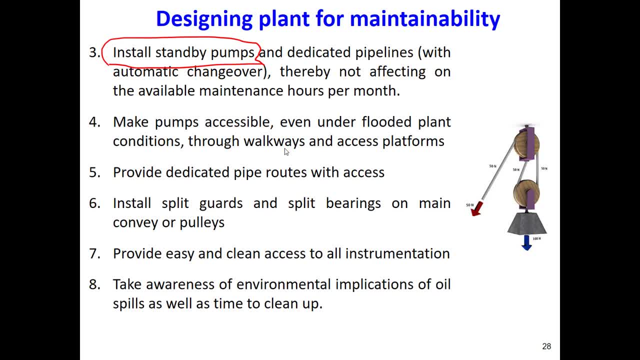 So when the pump needs maintenance, we switch to the other pump, to the parallel pump. So we do the maintenance, We fix it, We switch back to the main pump. So we need to design such things in the process And even the pipeline. you know we have to dedicate some pipeline that is used for purging, for maintenance, for, you know, this kind of work. 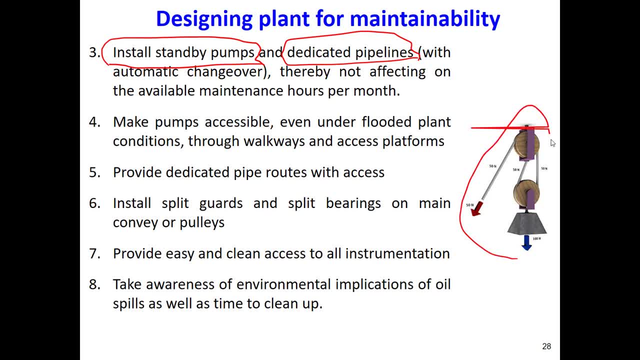 Then you know, as I said, we should design device. I mean lifting device, moving devices to move the equipment, to lift them. you know like we have to relocate them To be accessible. Those are the things that has to be.